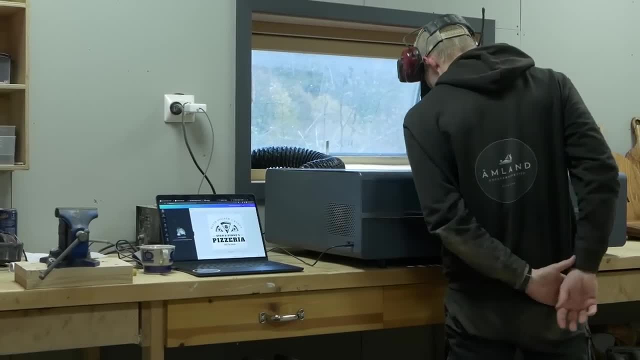 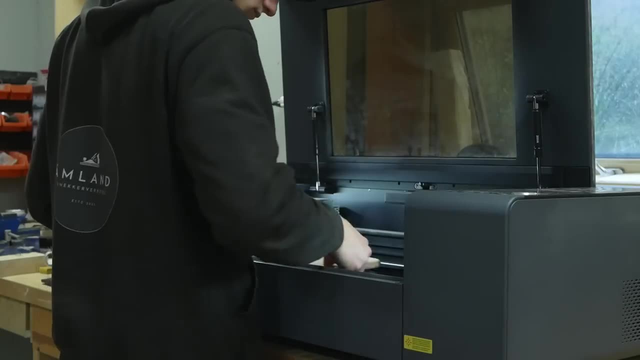 I'm going to show you how to make these products. So a little over a month ago, I got this laser. I started playing around with it, I made some products and I posted one single story on my Instagram, which only had like 200 followers at the time. And from that story I got my first four sales. That's when I realized I was onto something, So I kept posting and the sales started coming in like crazy. Fast forward to one month later and I've sold for $8,300. 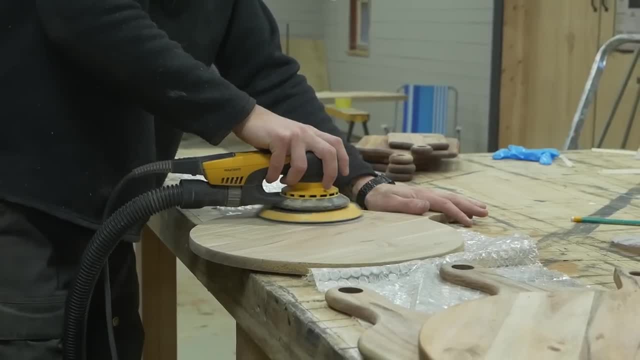 And I've sold for $8,300.. And I've sold for $8,300.. Now I have used one product a month later and I've sold for $8,300.. Now I have used one strategy in particular that I've never heard anyone else talk about. 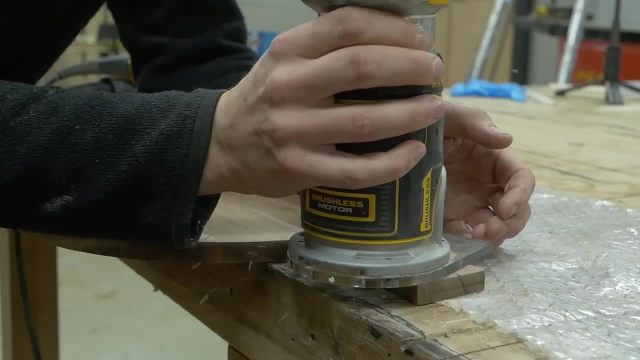 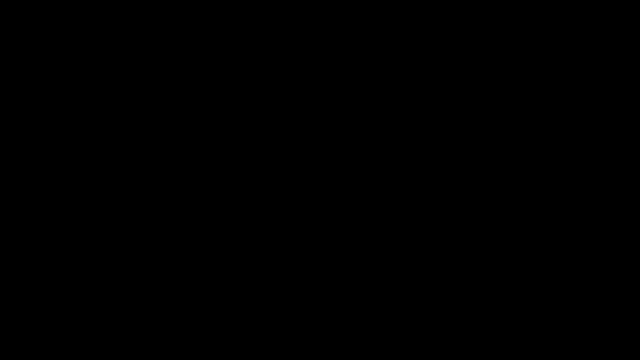 And it has given me half of the sales, And I'll share more of that later in the video. But first the question you've probably figured out by now: What products have I been selling? Good morning guys. It is a beautiful day here in Norway. 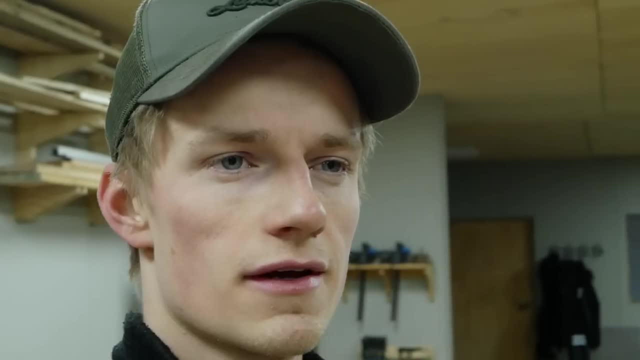 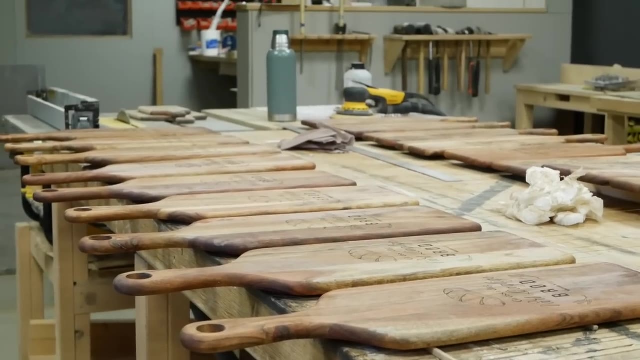 A little bit of snow- minus seven degrees Celsius- And it's a perfect day to finish up some cutting boards. So today I'm finishing up a batch of 60 cutting boards. 51 of them are for the same customer, 51 of them are for the same customer. 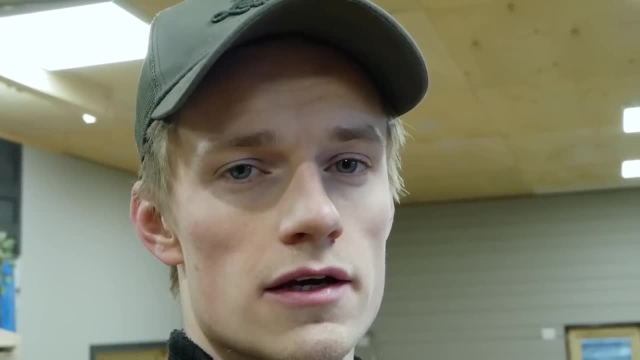 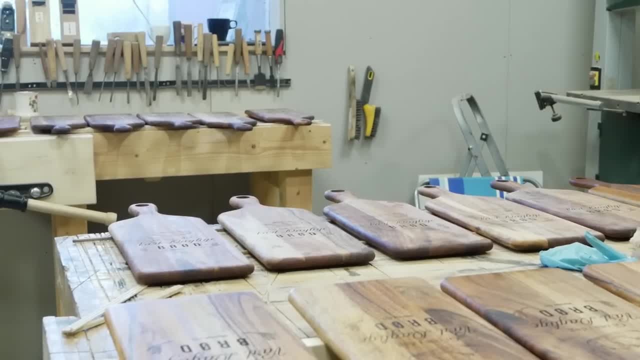 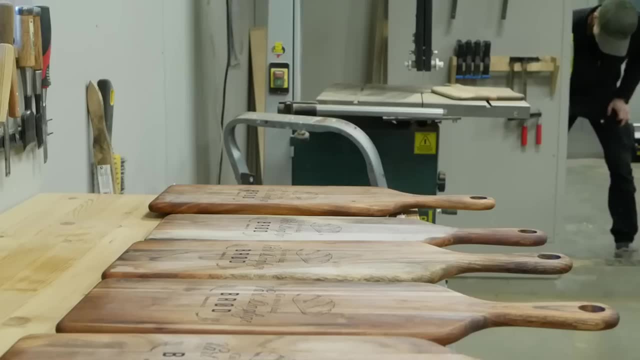 So this is what I'm making: Engraved cutting boards. I started selling them exactly one month ago And I've sold for a total of $8,300.. Notice that. that's not the problem, That's the profit. That's how much I've sold for in total. 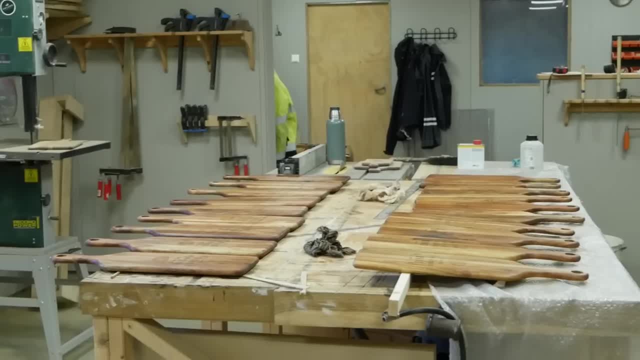 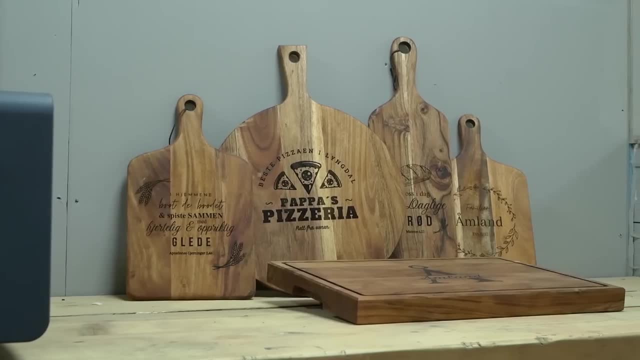 But I'll get into more details about that later in the video. So I've got a few different sizes on my cutting boards with some different engravings. Most of the cutting boards have a Bible verse on them, which definitely limits the potential customers. 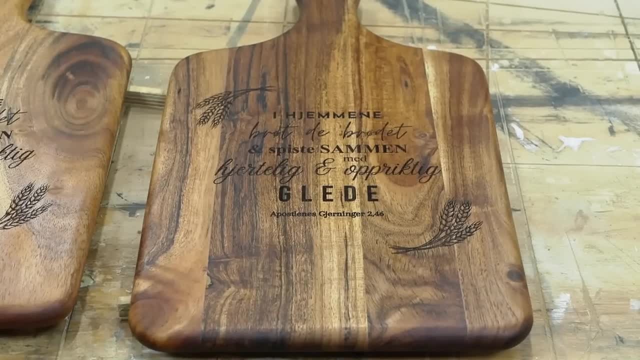 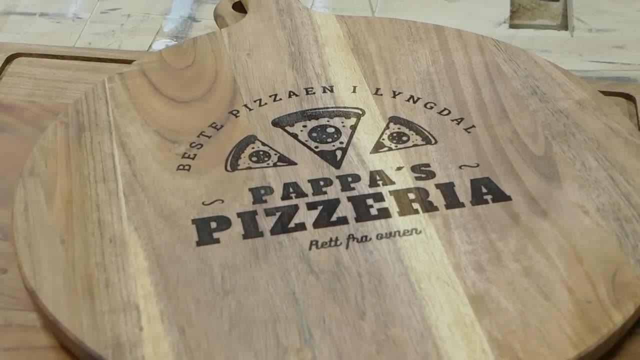 But I think that that's a good thing. If you try to reach too broad, there is a risk that you'll reach no one. I also made it possible for people to have a personalized engraving, But even though I charge a little more for that, it takes a lot more time. 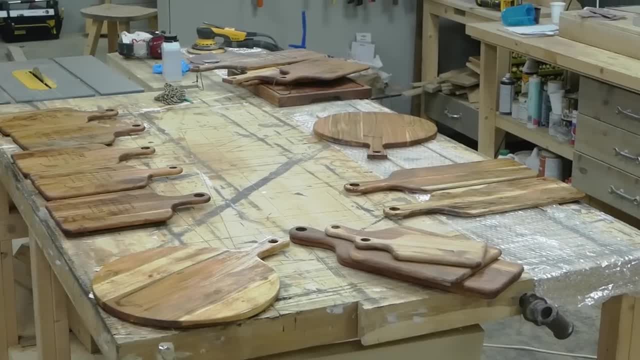 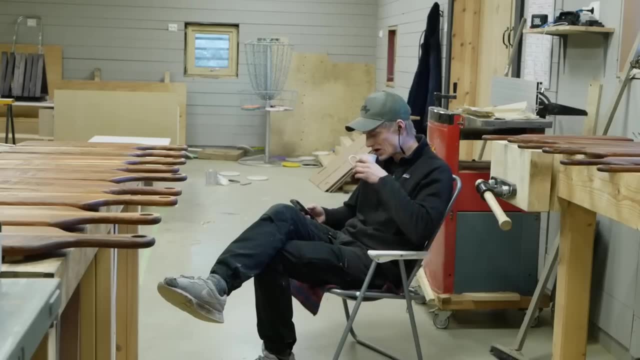 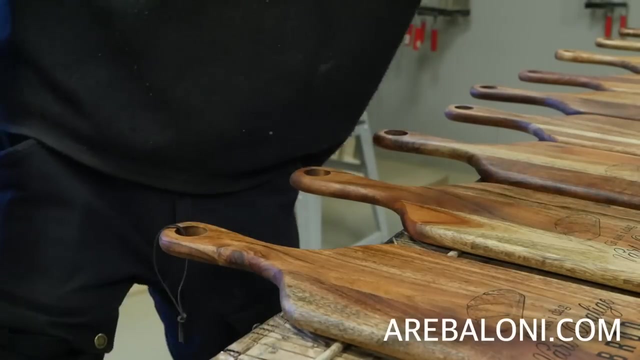 And I'm not sure if that's worth it for cutting boards. I'm from Norway and I'm selling in Norway, So all of my engravings are in Norwegian. But I have made English versions of all of my laser templates And, if you want to buy them, they are available on my website, aribolognycom. 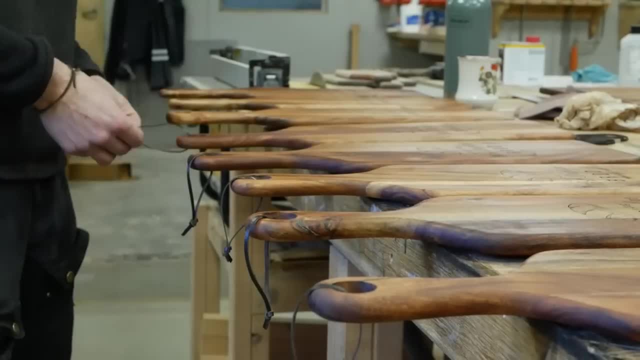 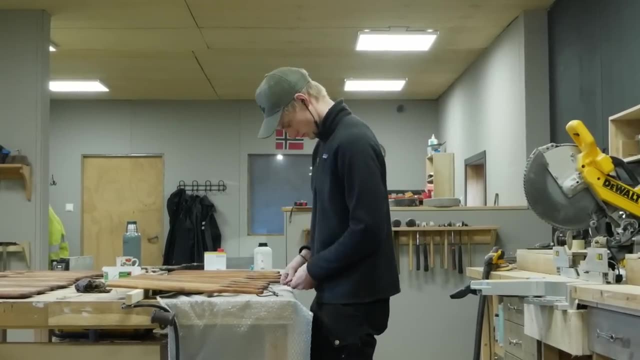 I've got to be honest. This almost feels like cheating, And the reason I say that is I don't even make the cutting boards myself. I buy batches of unbranded rough cutting boards, I sand them down, engrave them, sand them again. 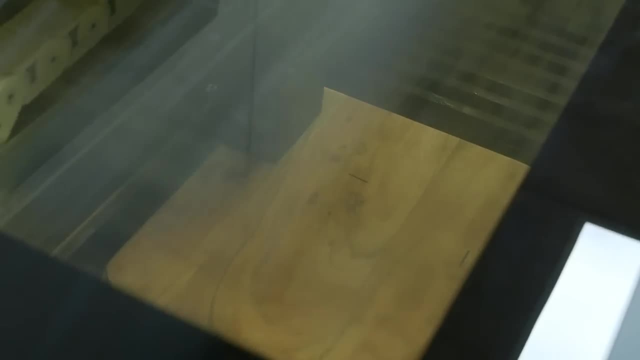 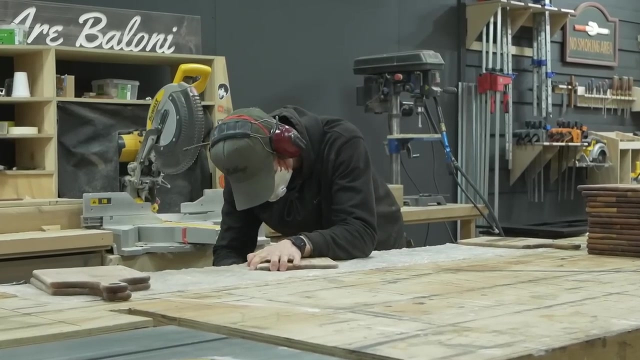 and then finish them and add a leather strap, And that's all I do. Of course, I could have made the cutting boards from scratch, but that would take a lot more time And I'd have to at least double the price in order for it to be profitable for me. 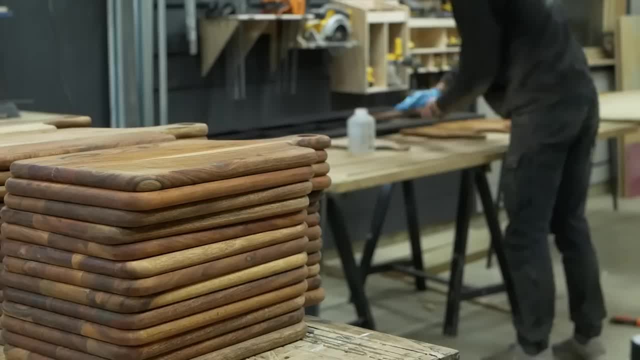 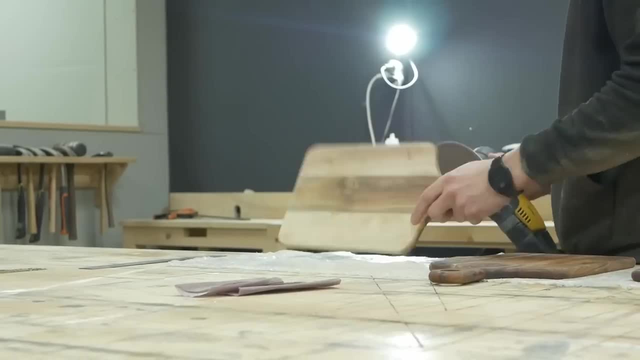 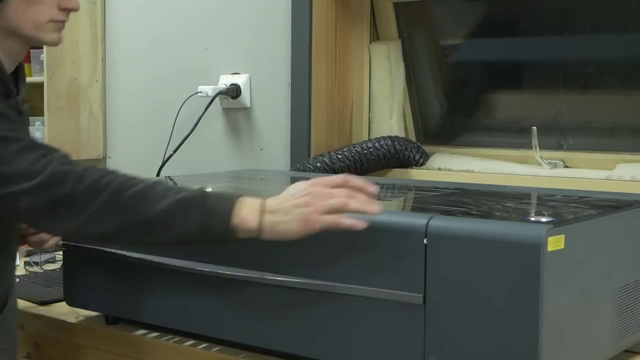 And it also requires a lot more tools and machines, The way that I do it now. all you need is a sander and a laser cutter, And that's it. These marks aren't examed right. We simply go through those marks. 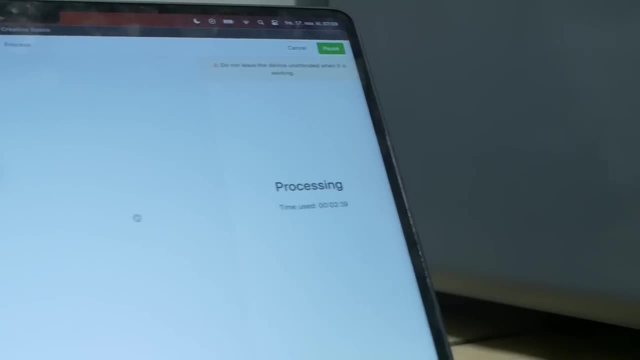 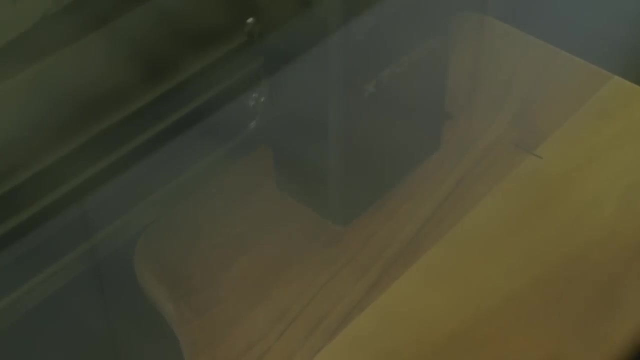 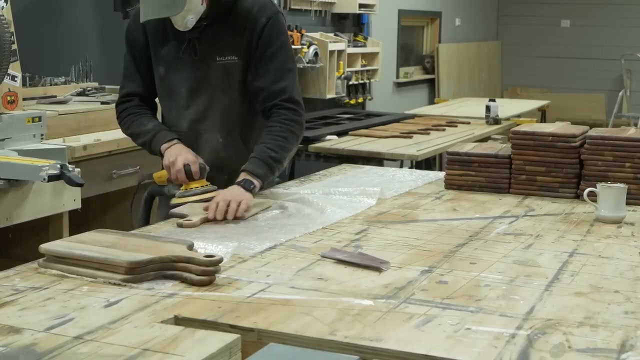 So it does look pretty good, Very delicious, But the encouragements are so small. Some of you may ask me how I prepare these. Well, the words I say are stronger. There's no link to науч. yes, But I say it hurts. 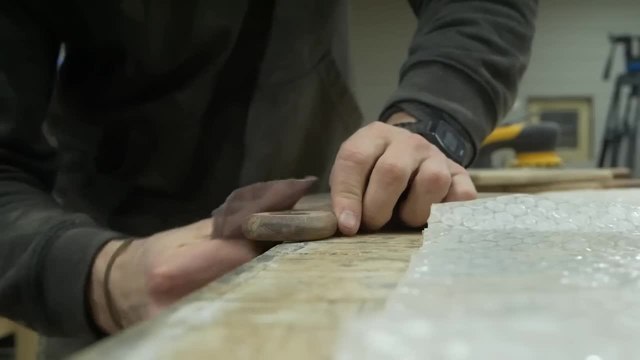 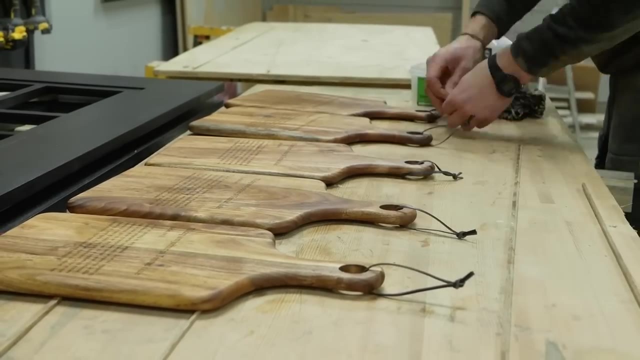 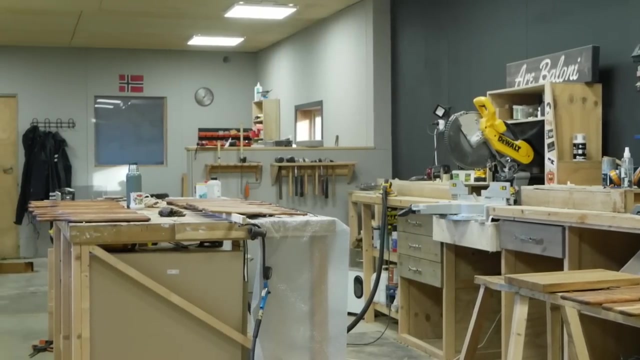 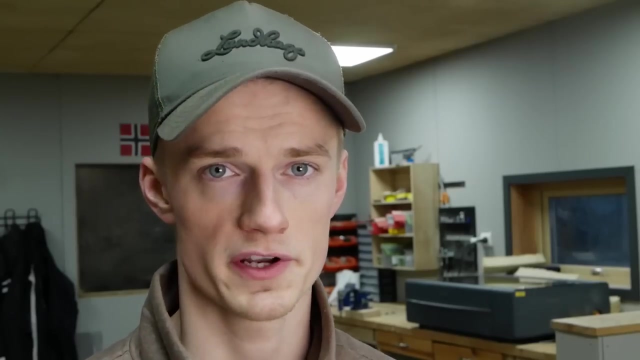 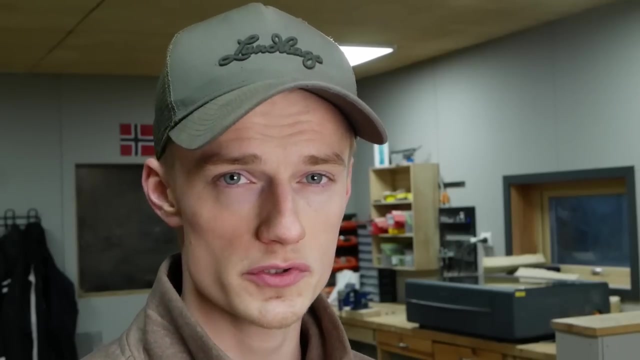 And it works. so let's take a look at how i managed to sell over 200 cutting boards in just one month. so i knew that i had a good product and now it was all about getting eyeballs on it. with a social media following of just 200, it's very limited how many customers you can get, and that is why i decided to. 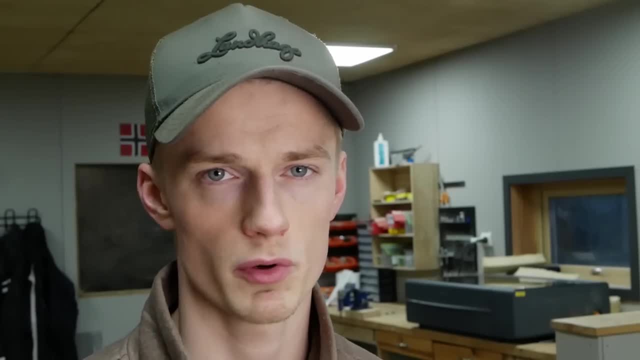 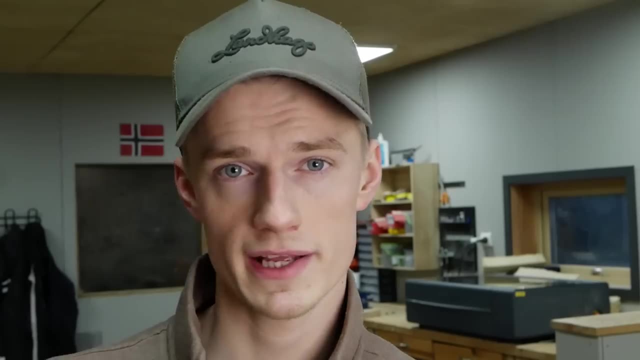 do giveaways. i did two giveaways during this month and they both did very well. just make sure you are giving away the actual products that you're selling and not something else. that way, people get to see your products and hopefully a lot of people will share it with this strategy, not only. 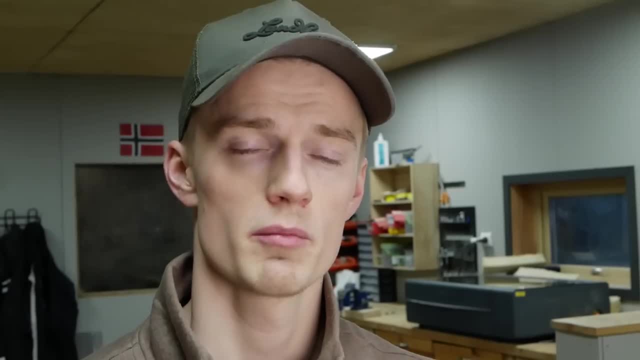 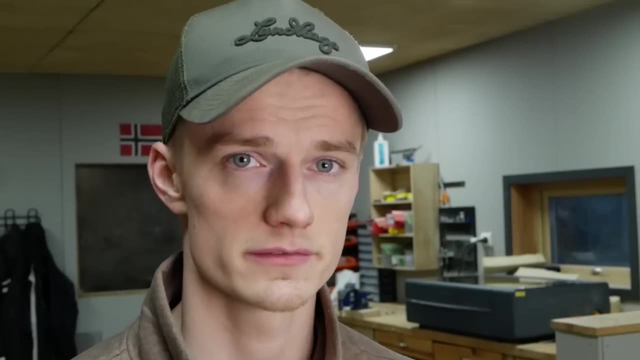 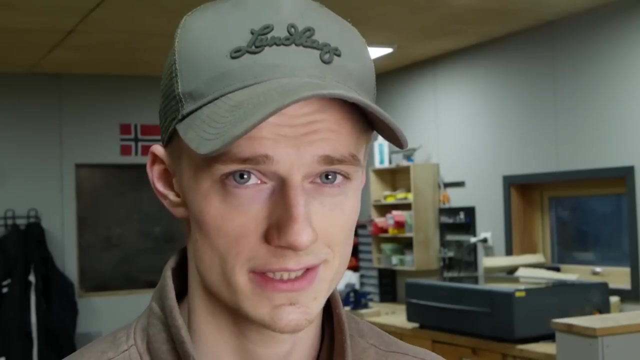 did. i get a lot of sales after the giveaway was done, but i also doubled my following, which has led to more orders for products that i will make later. here's a little pro tip: make sure you read the facebook or instagram guidelines for giveaways and follow those guidelines. i did not do that on the first. 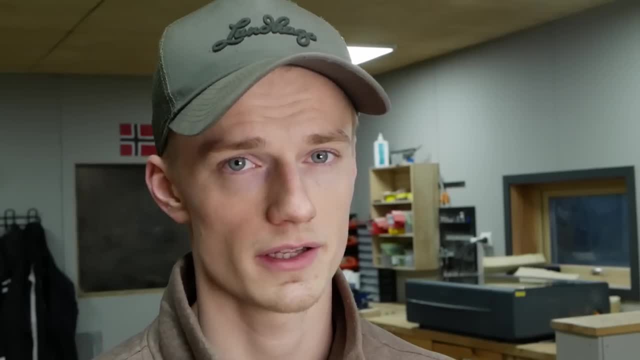 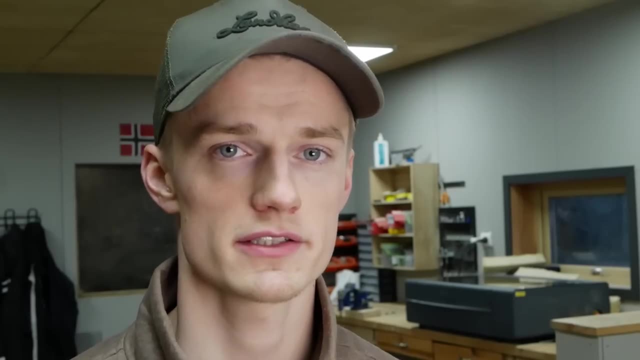 giveaway and i could have gotten into trouble, but luckily i got away with it. the second strategy is one that i haven't heard anyone else talk about, but it got me most of my sales. getting customers who are buying one or two cutting boards is really nice, but it can also be very time consuming if 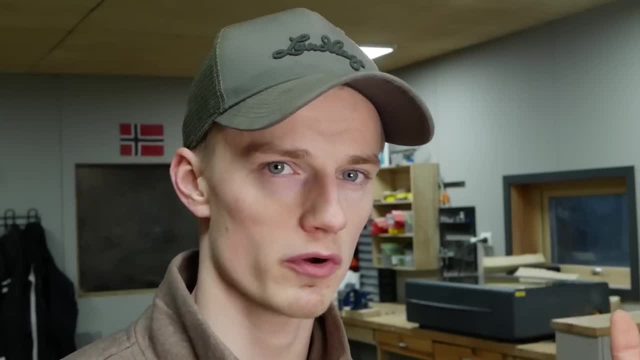 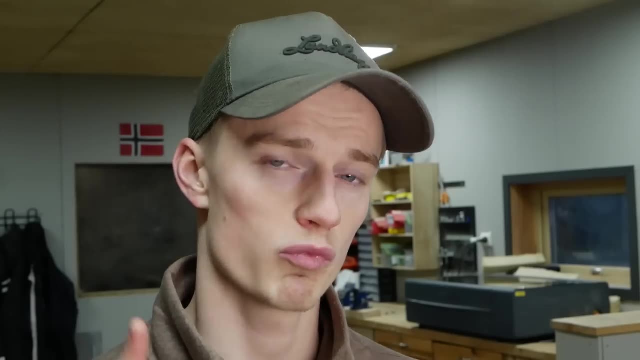 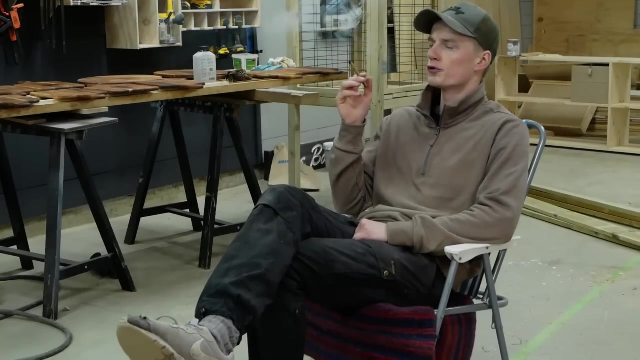 they're going to have different prints. so you have to stay in control of what type of board they want, what type of print they want, and you also have to deal with a lot of customers. there's a lot less headache if you can get one client to buy many cutting boards with the same print. so one day i was sitting in my shop doing 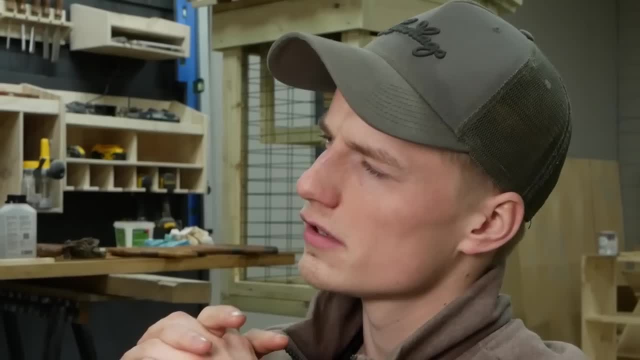 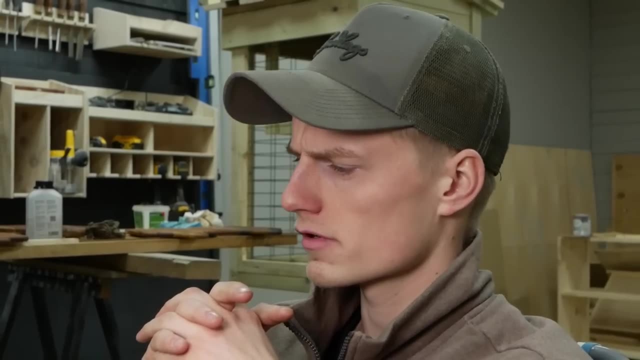 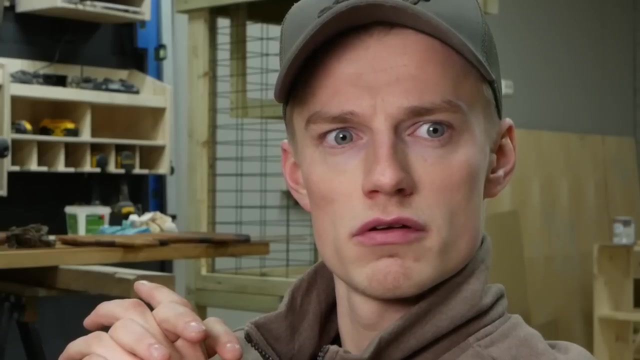 absolutely nothing when i started thinking. it's soon christmas. most companies give christmas gifts for their employees. i'm selling cutting boards with bible verses. what sort of company would give that to me? itаны examples. let's see what i got from christian private schools. so i grabbed my macbook and found a list of all the christian private schools in my 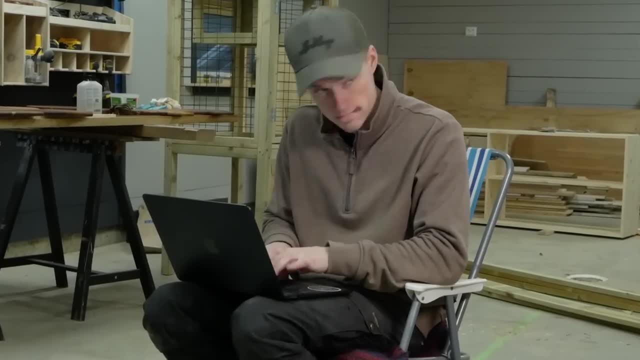 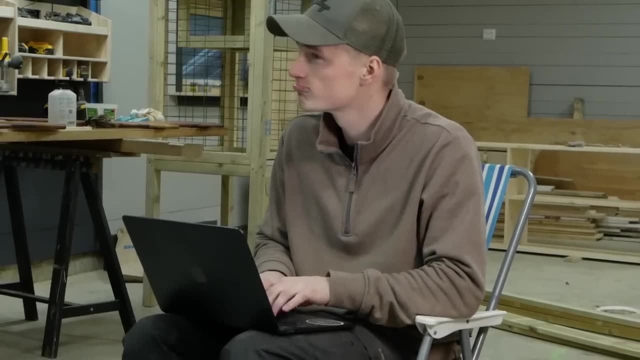 area turns out there are about 20 of them. i sent them an email. i gave them a short introduction and said: hey, i've got an idea for a christmas gift that you can give to your employees. i gave them three offers with discounts and some pictures, and sent it away. after a few days i finally got 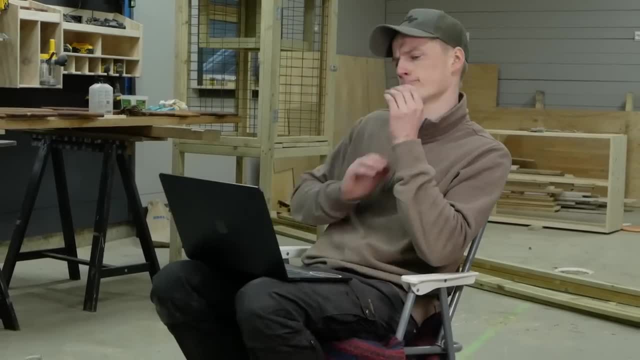 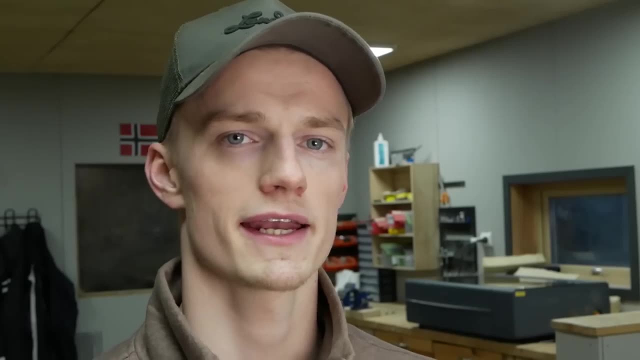 a reply and i managed to get two big orders and in the end i was win okay. so when i had them i went to some virtual neurocontext alliance and actually friendl wegen of a total of 96 cutting boards. And now in month two I got another one at 44 cutting boards. 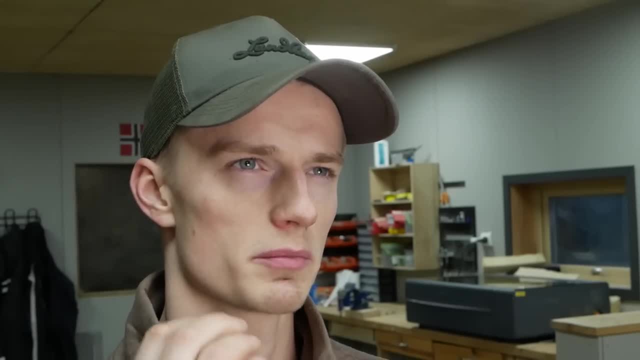 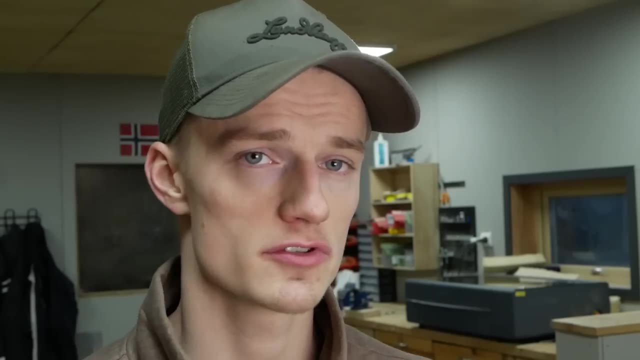 So try to think about. are there any companies who would be interested in buying a large batch of your product? Maybe like a car sales company? they'll usually give a gift to their customers when they're selling a new car. Could you be the one making that gift? 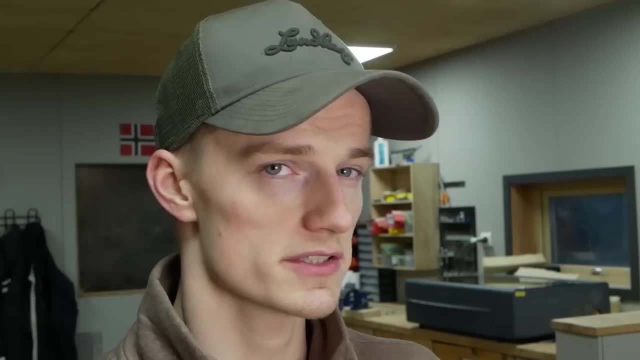 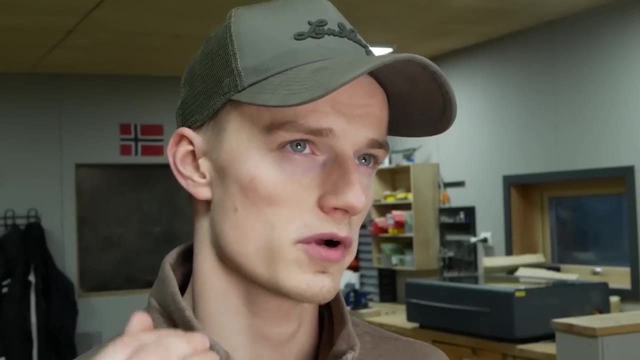 and selling it to the car sales company. The same goes for real estate. You'll usually get a gift from the real estate agent when you are buying a new house, So try to think of companies who would want to buy a large batch of your products. 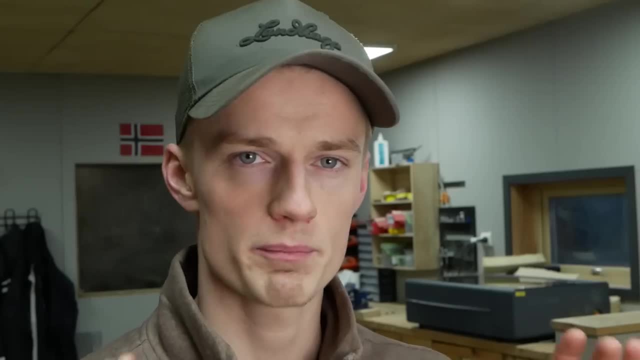 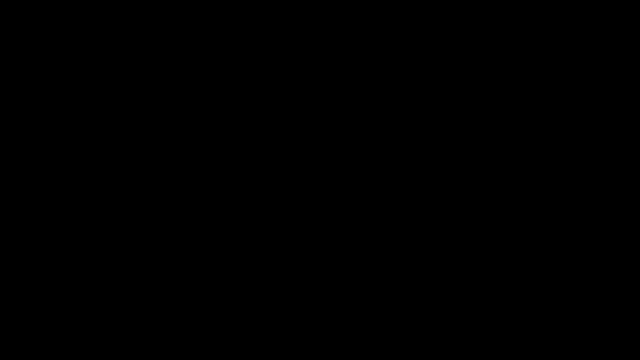 That is where the big money is. That's where you can just make a bunch of the exact same products and you can make them a lot quicker. So now let us take a look at the exact numbers. My total income was $8,300.. 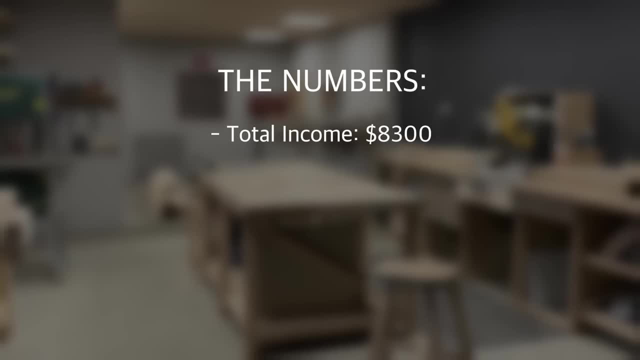 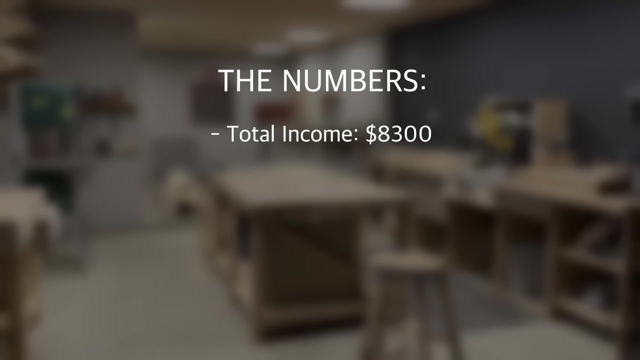 The prices for the cutting boards varied from $40 to $90 per cutting board, But for the clients who ordered a large amount, I gave them some discounts And for the expenses which includes the cutting boards, the finish sandpaper and the leather straps.